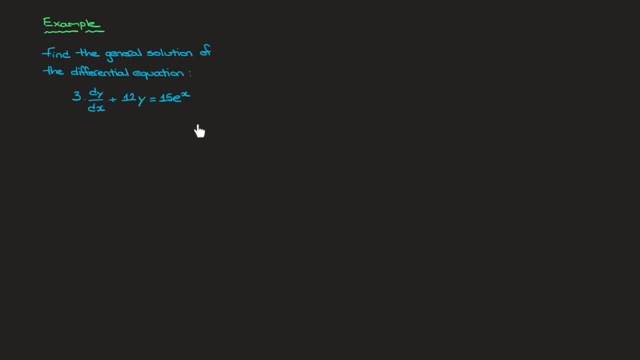 we can tell right away that we're dealing with a linear differential equation here simply by comparing it to what I would call the standard linear ordinary differential equation. And the fact that it's a linear differential equation is exactly what tells us, or what should trigger us, to use the integrating factor, And the method for doing so can be summarized in three. 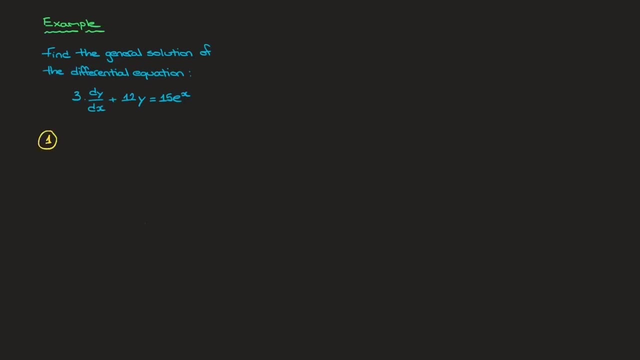 steps. The first step, step 1,. we need to make sure that our differential equation is written in the form dy dx plus 12y, dy dx plus p of x times y, which equals to q of x. In other words, we need to make sure 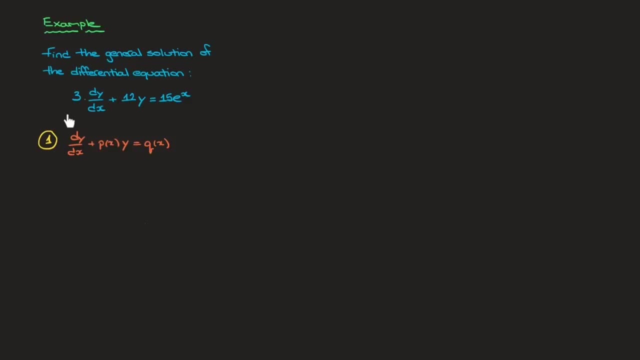 that there's nothing multiplying the dy dx. So, looking at the example we have here, we need to get rid of this 3. And for that all we have to do is divide both sides of this equation by 3.. So that would be dy dx plus 12 over 3, which is 4y equals to 15 over. 3.. So that would be dy dx plus 12 over 3,, which is 4y equals to 15 over 3.. So that would be dy dx plus 12 over 3,, which is 4y equals to 15 over 3.. 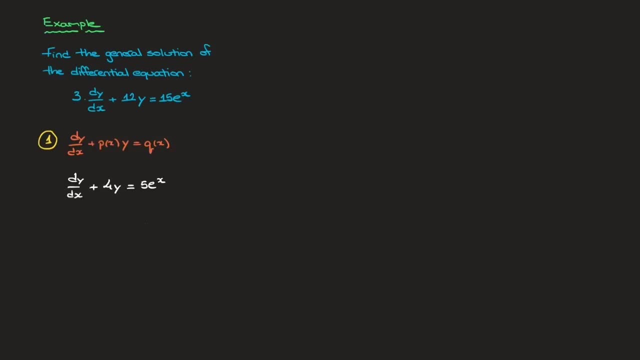 So that's 5e of x And that's our first step done, where all I did was divide every single term by 3.. So we move on to step 2. And in this step we need to find the integrating factor. So I'll just write: find integrating, that's integrating factor. We usually call 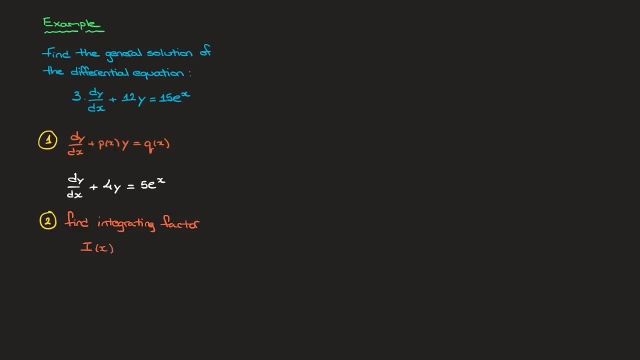 the integrating factor, capital I of x, And to find it we use the fact that it's equal to e of the integral of p of x, Where, to be clear, p of x is the function multiplying the y inside our differential equation. So in this example, p of x is just 4.. And don't let the fact that there's no 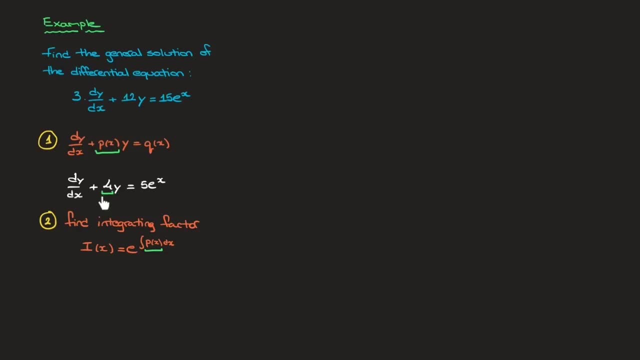 x here, bother you. There is nothing wrong with having a function simply equal to 4, or any other number. That being said, I carry on. I of x is therefore equal to e of the integral of 4.. And that leads to. 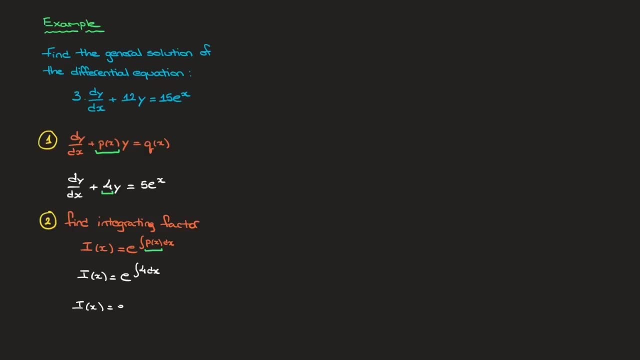 I of x equals to e of 4x. Notice here that I'm not writing any constant of integration. In fact, as soon as we look for an integrating factor, we'll always ignore the constant of integration. And so that's step 2 done And we move on to step 3.. And in this step we start by multiplying the. 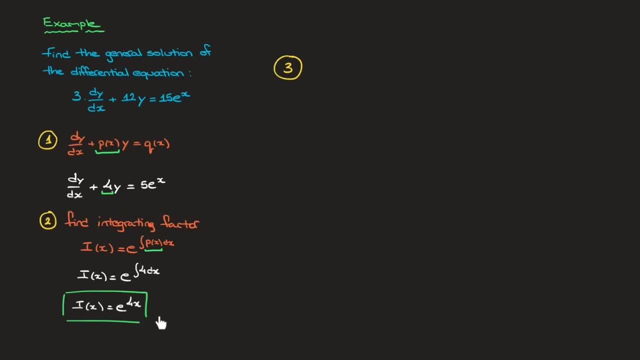 differential equation we have here by the integrating factor we just found. Once that's done, we'll use the fact that we have the integral of 4x, And so that's step 2 done And we move on to use the product rule and solve the equation. So I'll just go ahead and write: multiply, multiply. 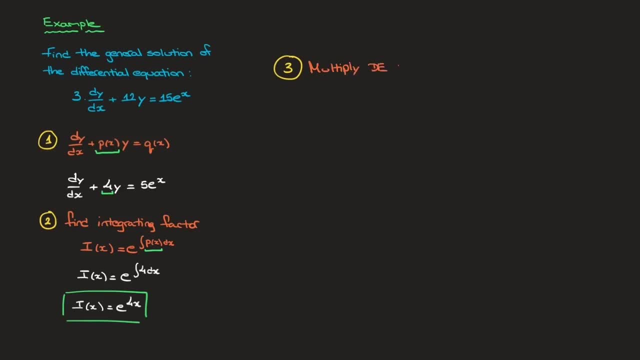 dE, as in differential equation, by the integrating factor I of x and use the product rule. So I'll just write: use product rule, product rule and solve All right. so multiplying this differential equation by e of 4x leads to e of 4x. 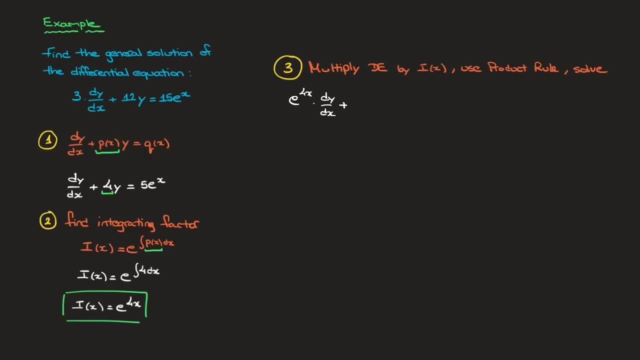 So e of 4x times dy, dx plus e of 4x times 4 times y, which equals to e of 4x times 5 times e of x. And on the right hand side we notice that the product of e of 4x and of e of x will turn into: 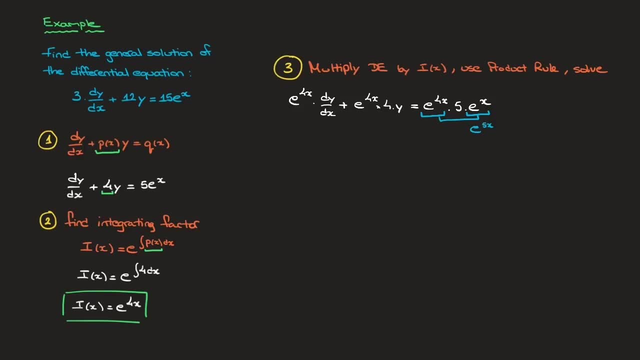 e of 5x, And so we can write this equation as: e of 4x times dy dx plus 4x times dy dx, And so we can write this equation as: e of 4x times dy dx plus 4x times dy dx. 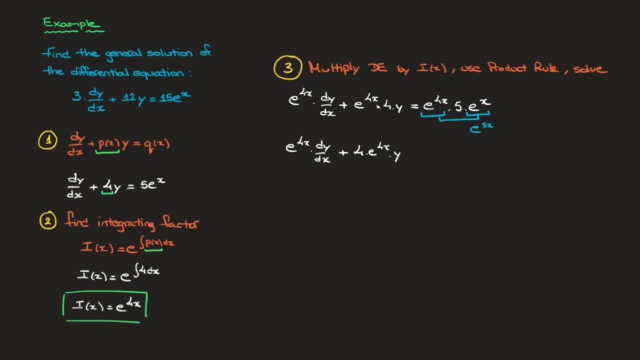 4 times e of 4x times y, which equals to 5 e of 5x. And now for what is perhaps the most important part. If we look at the left-hand side of this equation, we can see the whole idea behind using the integrating factor. 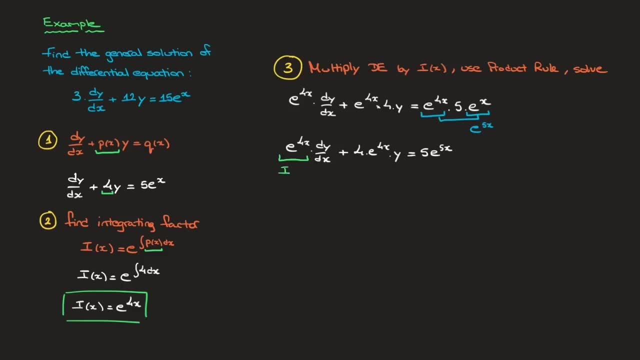 Indeed, we know that e of 4x is the integrating factor, that's i of x. but on top of that we notice that 4 times e of 4x is the derivative of e of 4x, In other words, it's di dx.